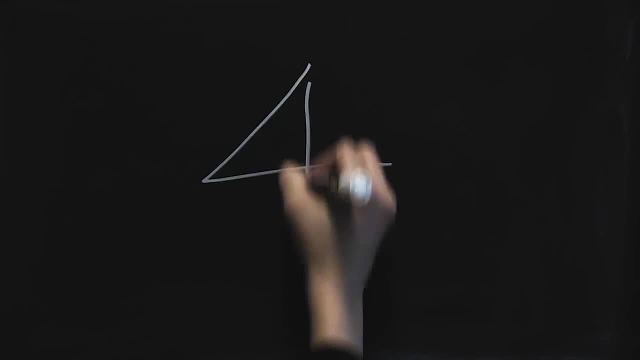 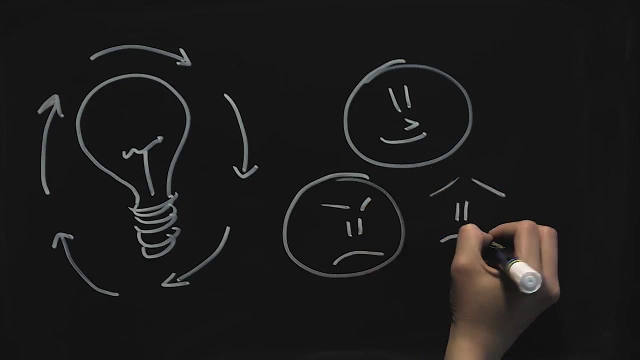 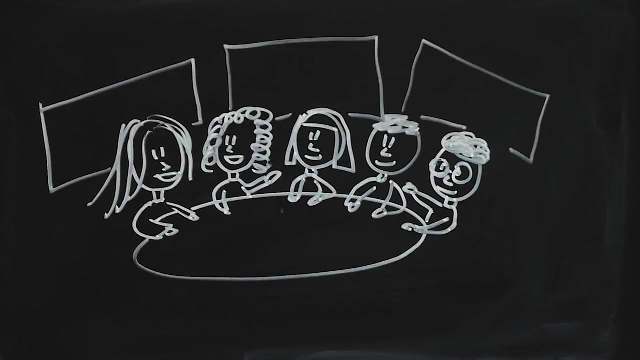 importance of the environment in the New Zealand culture. Four: it's actionable by working in complement and enhancing practices like design thinking, user experience or organizational development. When we studied financial depth and technology solutions for Harmony New Zealand, our observation work landed, amongst other deliverables, in user experience maps and 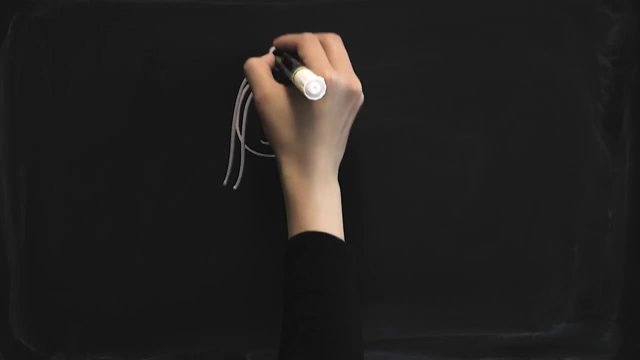 was used alongside as a design thinking sprint. If this makes you curious to know more about, If you're curious to meet us or work with us, send us an email and we'll take it from there. 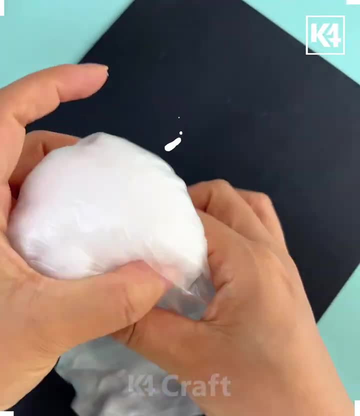 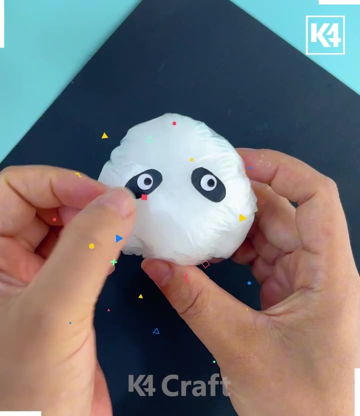 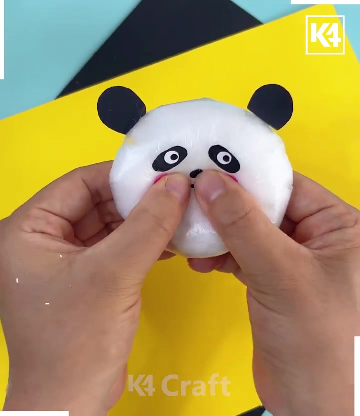 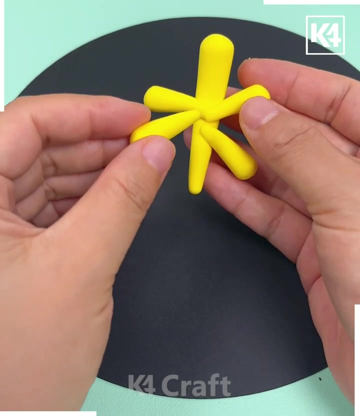 Hello everybody, Welcome to our Facebook page. Take a polythene like this and fill it with cotton and tie a knot at the end like this. You can also use a thread or rubber band. Then we are going to paste eyes of the panda. We are making a cute little panda. Paste its ears and look: your squeezy panda is ready. Let's make this cute little turtle For that. remove the seed of the peach. We are going to make the shell later. Now make the head and legs of the turtle using this yellow clay. Make the shell and draw its eyes and look: it is ready. 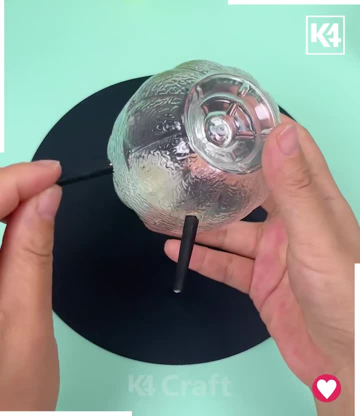 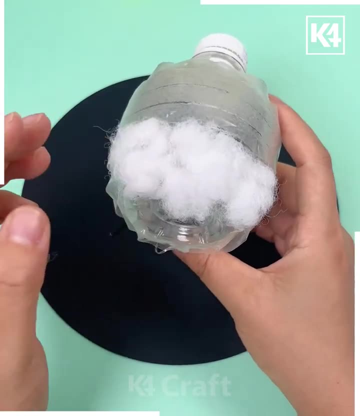 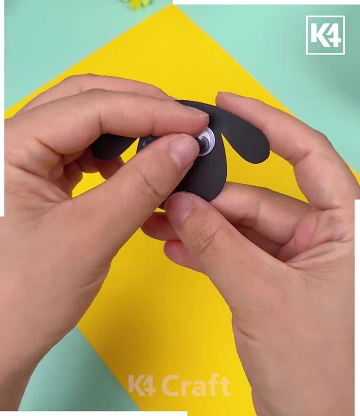 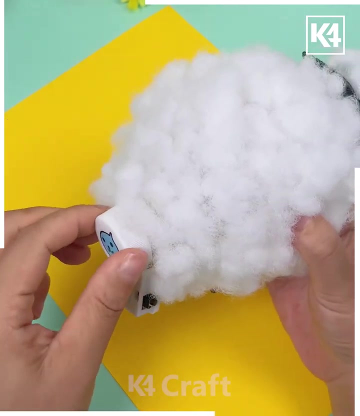 Let's make this glowing sheep. For that you need this type of plastic bottle. Now we are going to make the legs of the sheep. Paste all of them like this. Now cover the bottle with double sided tape and paste these different cotton balls around it. Cover the ball completely and look it is ready. Then we are going to make the head of the sheep. Paste googly eyes and look it is ready. Now put fairy light inside it like this, and look: your glowing sheep is ready. Look at this cute little toy. First we are going to make a 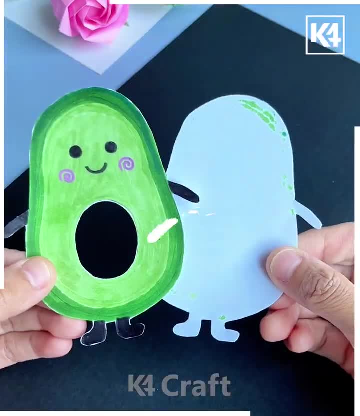 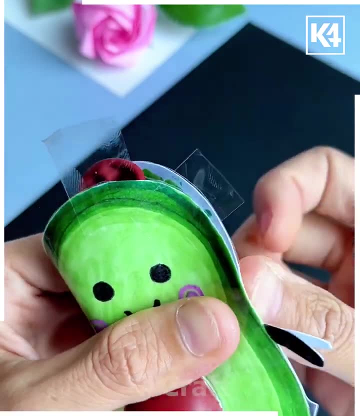 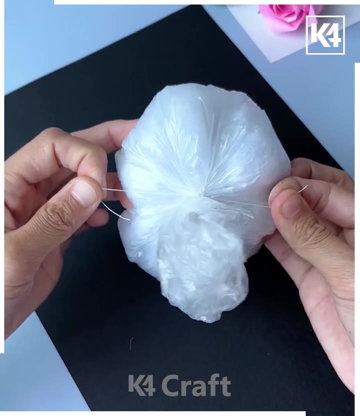 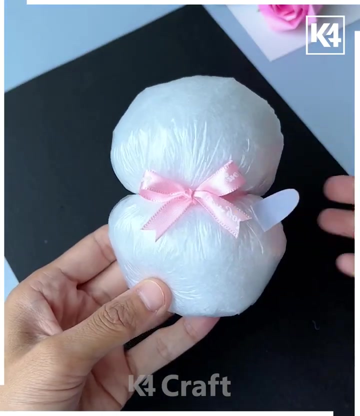 shape of avocado and make its eyes Color it like this. Now make a hole in the center. Paste cello tape on it. Now we are going to put this balloon inside and cover it from its side like this, and look, it is ready. We are going to fill cotton inside this transparent sheet and tie a knot like this. Cut it. Now we are going to make holes inside it, and then we are going to make two partitions. Now paste eyes and hands and ears and look, your squeezy bunny is ready. Thank you so much for watching this video.